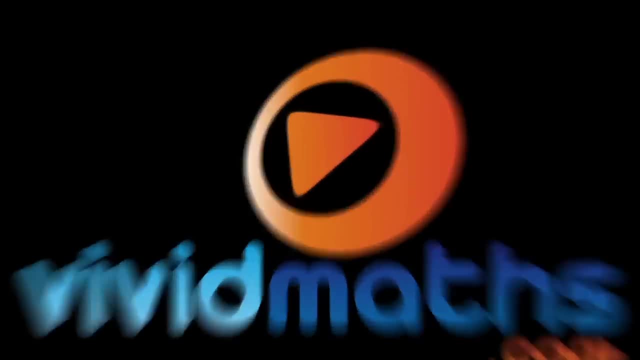 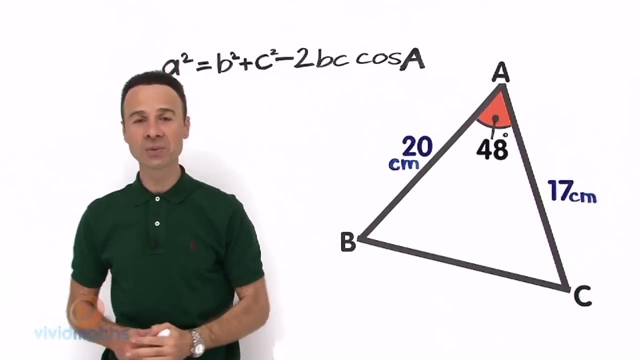 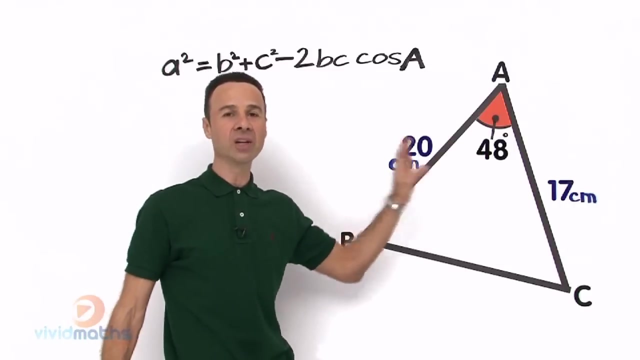 We are going to take this in two stages. first I am going to introduce the formula which is written up behind me, and then I am going to show you what each angle and length refers to in which part of the triangle. then we are going to substitute, drag and drop into. 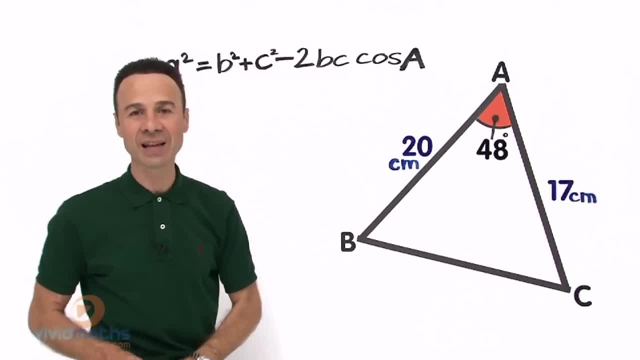 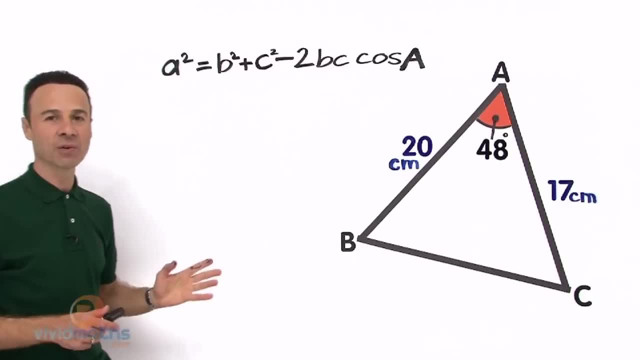 the formula and we are going to work out and come up with the correct answer. So let us start off with stage number one. let me introduce to you what each part of the formula are. So let us have a look. here we are looking for the length, little a why. 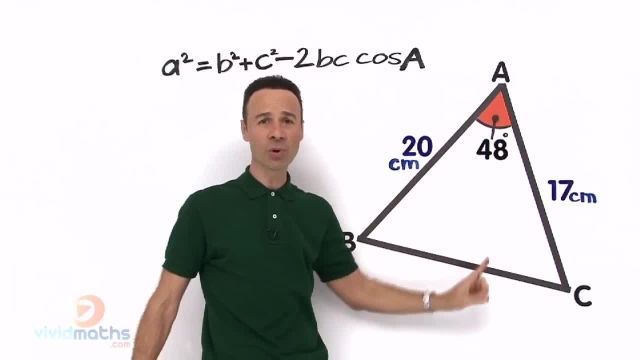 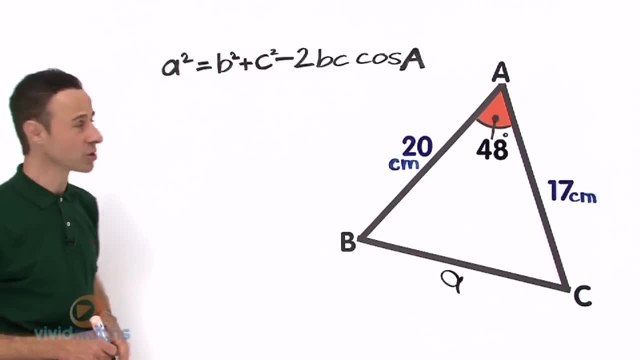 Because it is opposite capital A, which is the angle, 48 degrees. so we are looking for this little a here. let me write it down here: right there, there is our little a. that is what we are going for, and here is how the formula looks like. It is a squared equals. 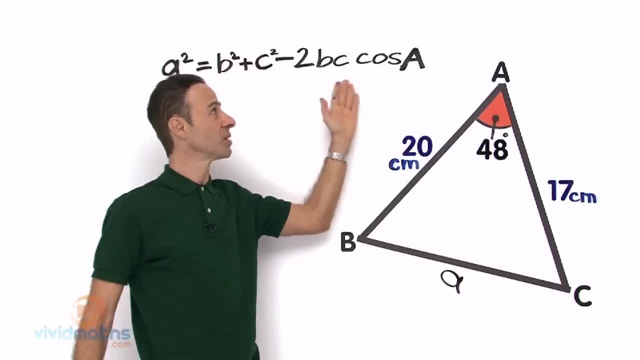 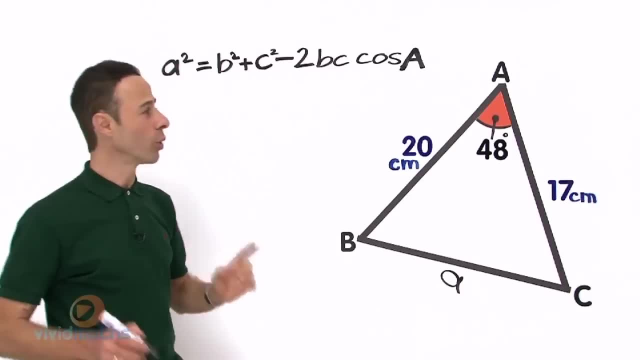 b squared plus c squared minus 2bc cos a. now that is very long and lengthy. It has got a lot of carriages. it is a very long train and when we take the appropriate numbers, the correct numbers, and put them in there correctly, it is all just drag and 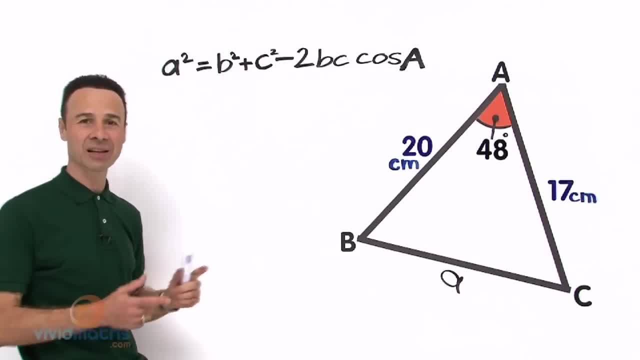 drop and it comes up rather easy. So let us start to look at, and take a closer look at, what each letter refers to here, what each pronoun refers to. Well, as I mentioned earlier, little a refers to the length directly in front of the 48. 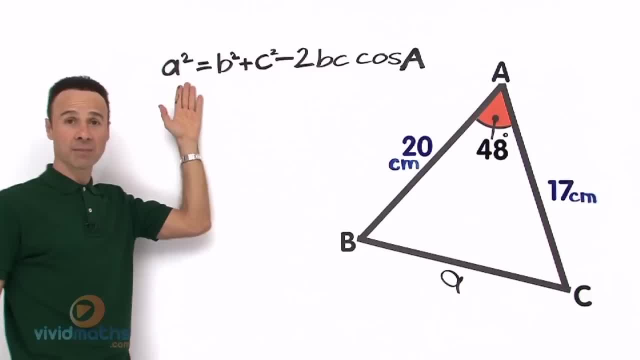 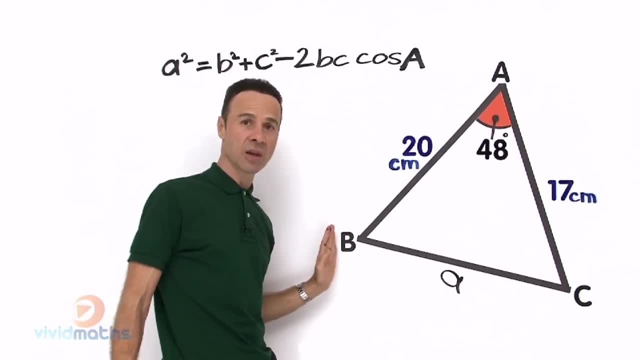 degrees. capital A- Now, that is what we are looking here. right A, that is what we are looking for Over here. we got the little b and the little c. where are they? Well, capital B is down here, so therefore, directly opposite will be. 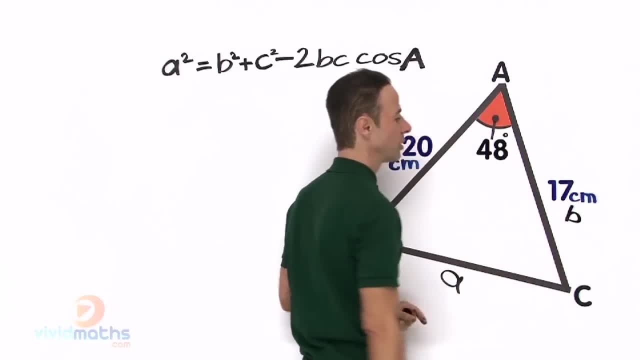 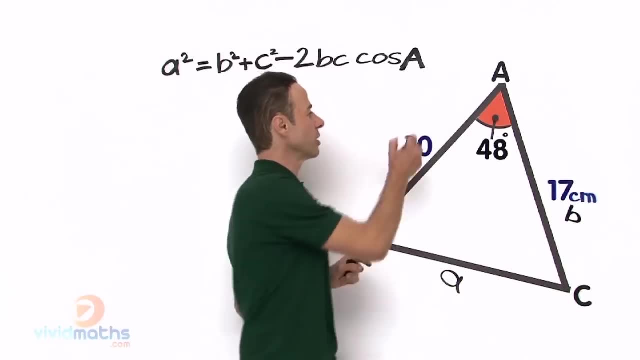 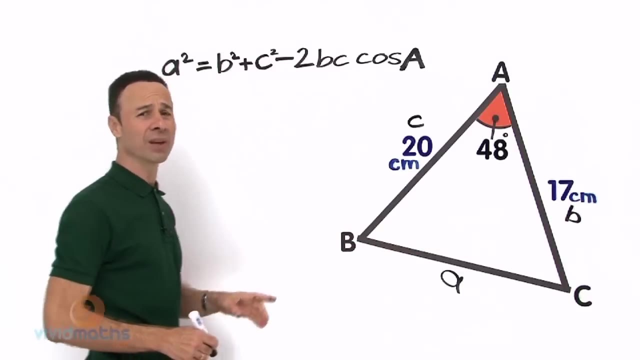 little b. so let me mark that out. There is our little b. Similarly, right opposite the capital C, the angle is little c, the length, and we will call this little c right there. Now that we have labeled our diagram, our triangle displayed right over there, we can. 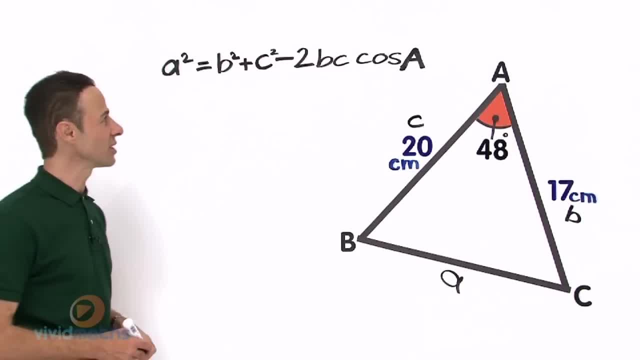 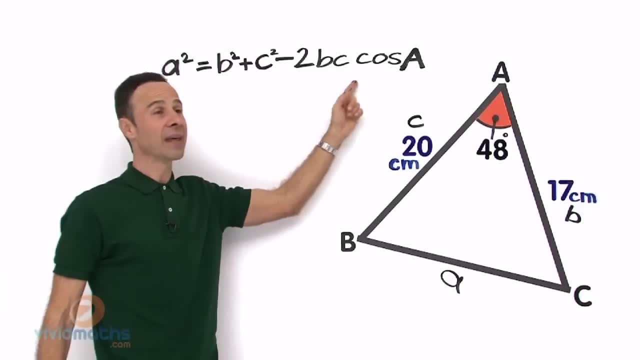 easily see where to drag and drop the appropriate numbers. So let us take another closer look at this. We continue with this very long formula Over here, we continue with minus 2bc and then we multiply. there is nothing there. it is actually a dot by cos of alpha and that alpha. 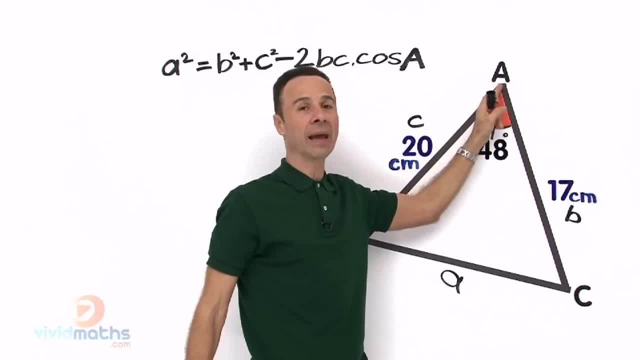 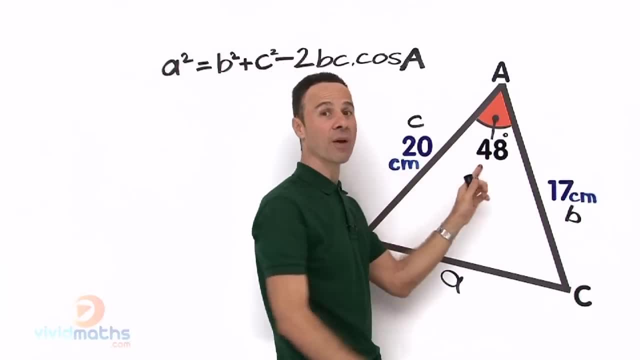 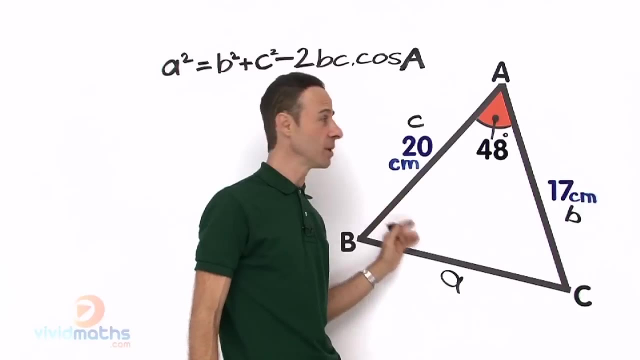 or A, that capital A is actually the capital A angle right here, 48 degrees. Okay, how do we know it is cosine rule? Very easy, it is cosine because it is cozy. we have an angle located amongst two lengths. We have the length c here, 20cm, and the length 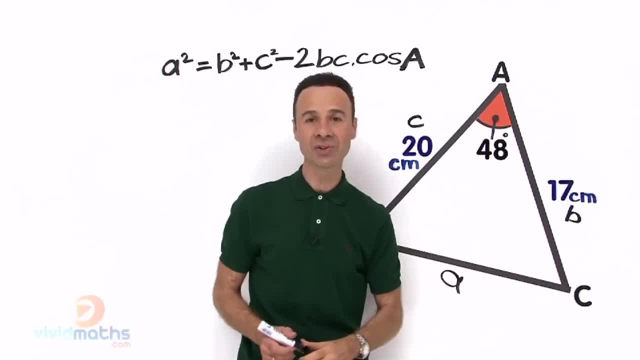 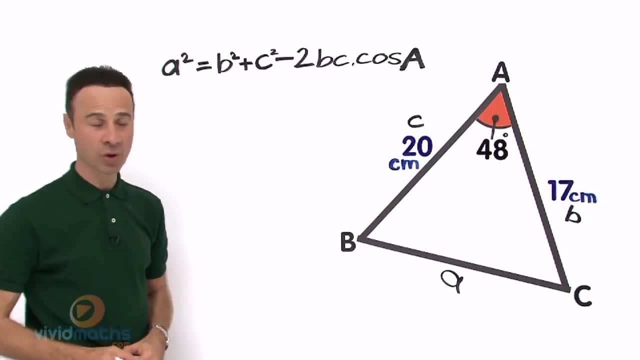 b here, little b, 17cm. So that is how we diagnose and detect whether or not it is a cosine rule or another one. So there is our formula. let us start to drag and drop the appropriate numbers into the formula. So let us start off. we have A squared equals. now we have little b, which is right over here. 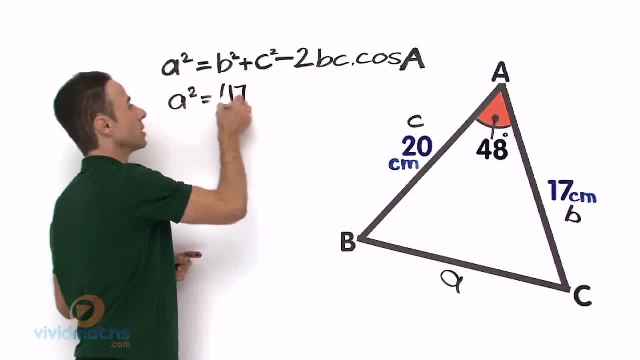 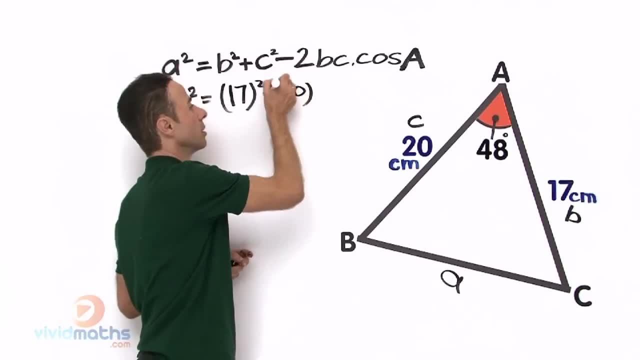 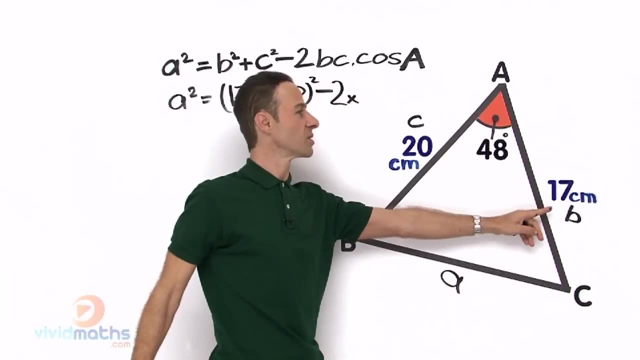 that is going to be 17,. 17 squared plus. then we have little c right there, that will be 20.. So we have b squared minus 2 times. now what is b again? Little b is 17,. so we go 17 times. 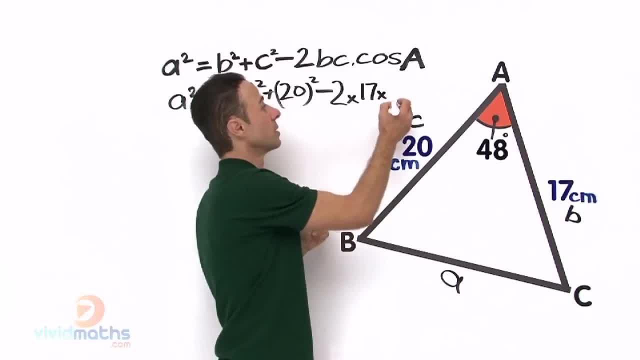 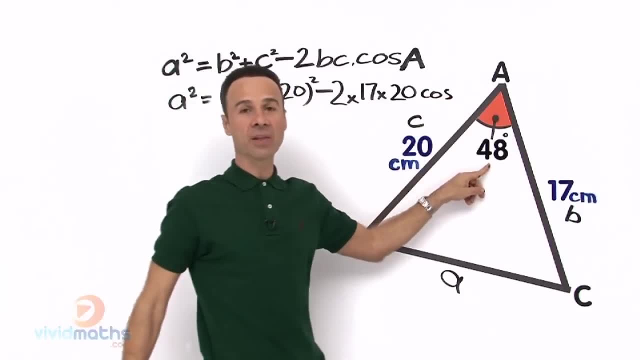 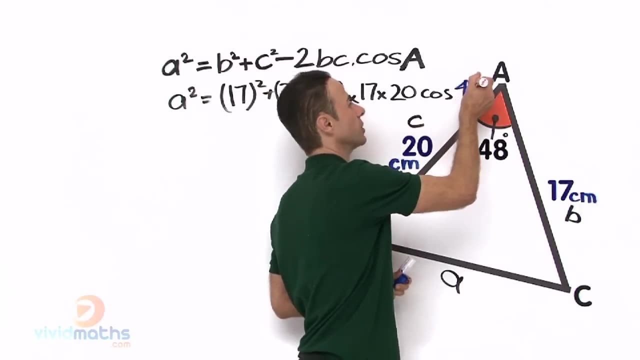 little c. there is a little c there. put it there times 20, and then we cos alpha or A capital A, that is 48 degrees. let me put that in blue right there: 48 degrees, that is 48 degrees. 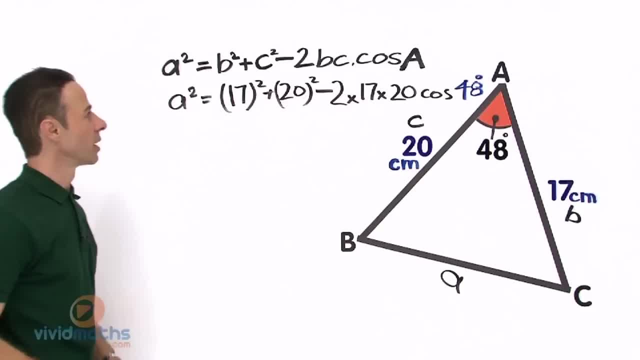 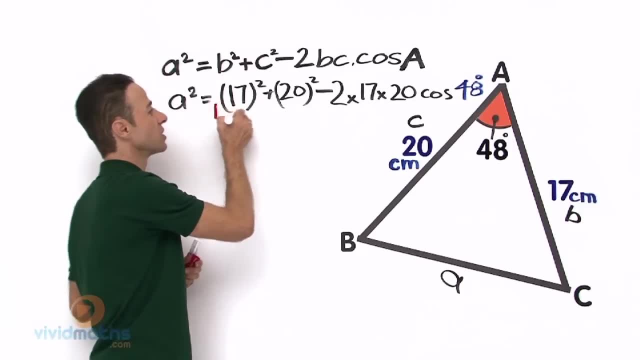 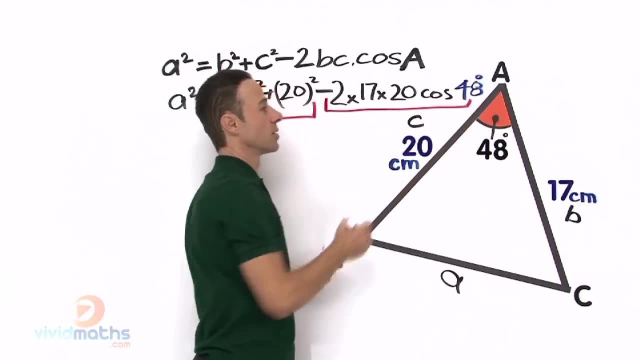 Now there is two sections to this formula and we are going to separate them in the two sections. The first section here is this part here, the 17 squared and the 20 squared. Then we have the other section here, right there, the second part of the train, or the second. 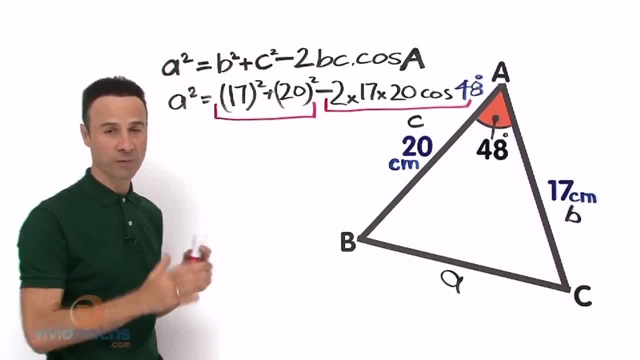 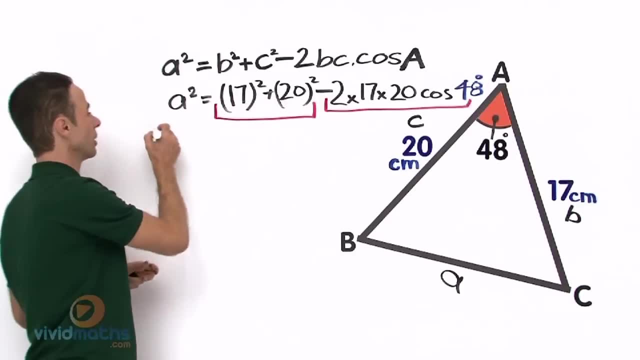 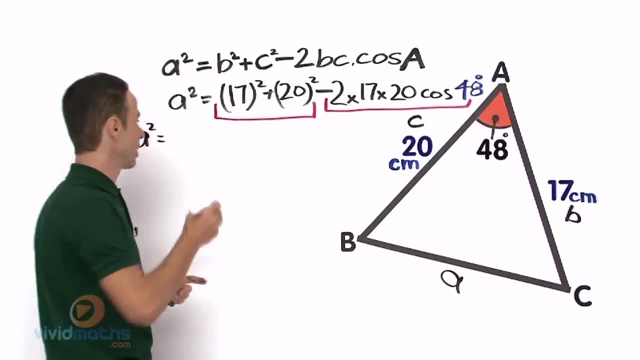 carriage, and we are going to keep them separate until finally we subtract one from the other because, as you can see, we have a minus sign there. So let us work out the section here on the left first of all. So A squared is equal to 17, squared in the calculator will yield 289 plus 20 squared in. 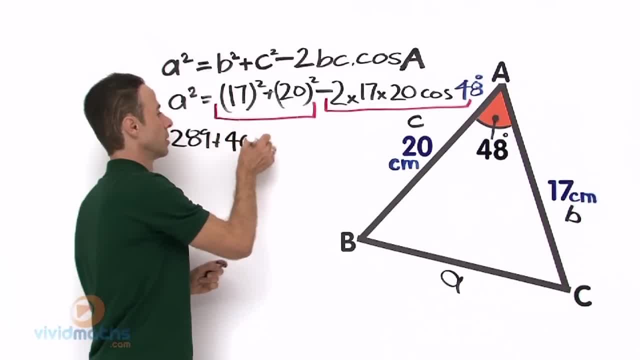 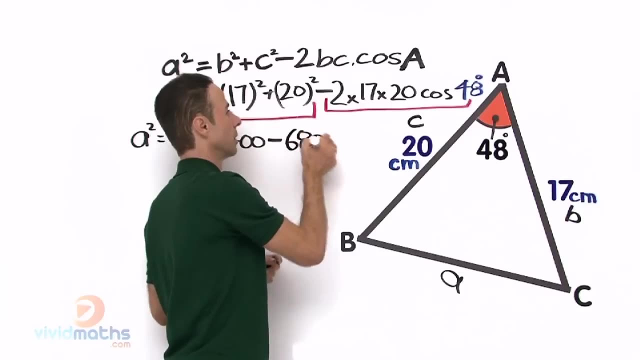 the calculator is 400 minus. let us go for the second part of the formula here. Now we got 2 times 17, times 20, now on your calculator, just that part will yield you 680.. So we got the two sections there. I am going to further simplify this section here in the 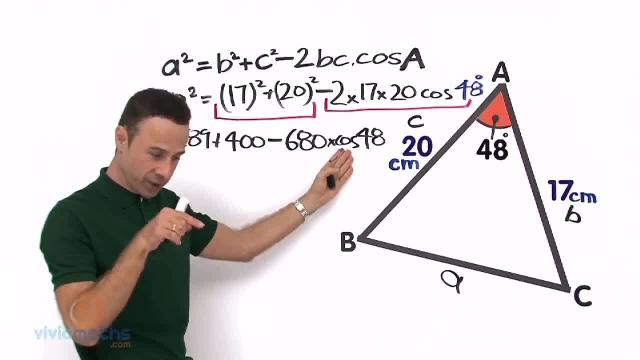 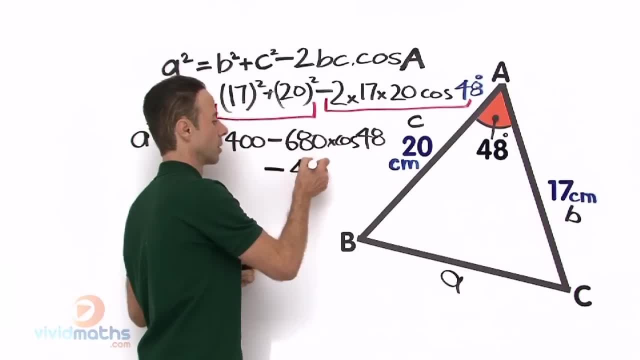 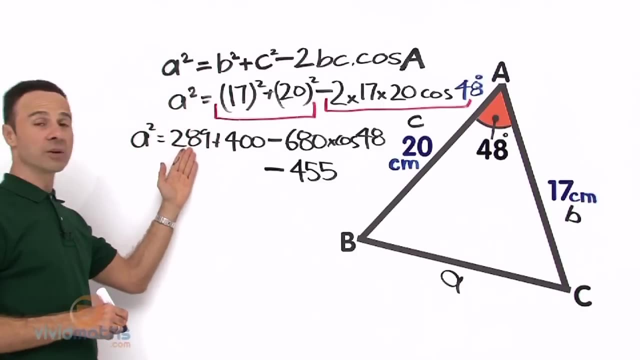 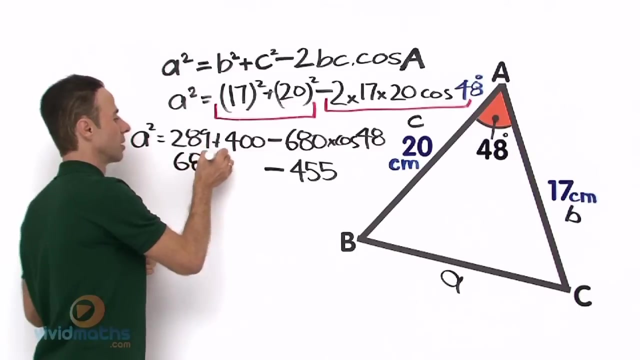 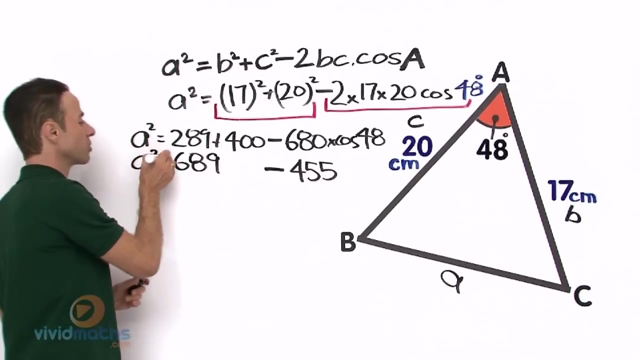 right, 680 times cos 48 on your calculator will give you a grand total of 455.. On the left hand side, if we add up 289 plus 400, that is going to be 689,, isn't it So? 689 minus 455.. Okay, so A squared equals. 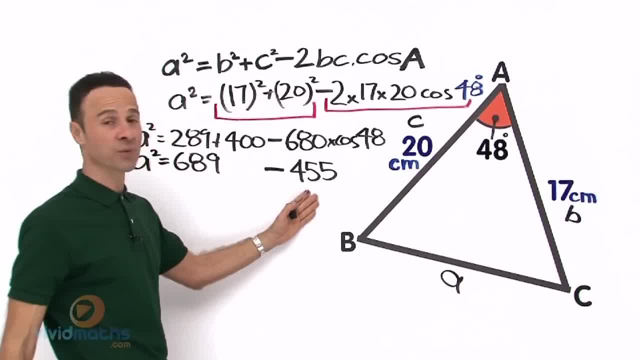 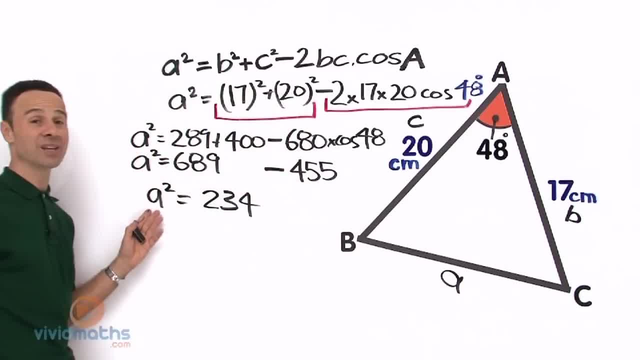 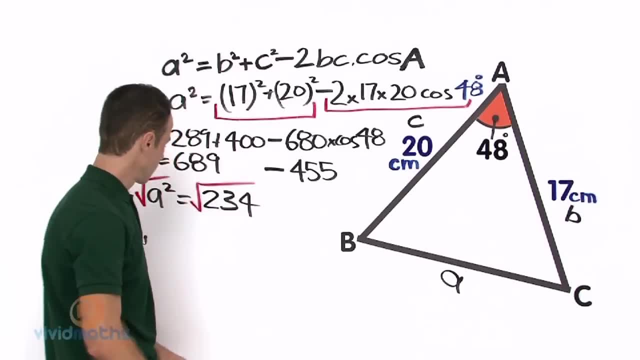 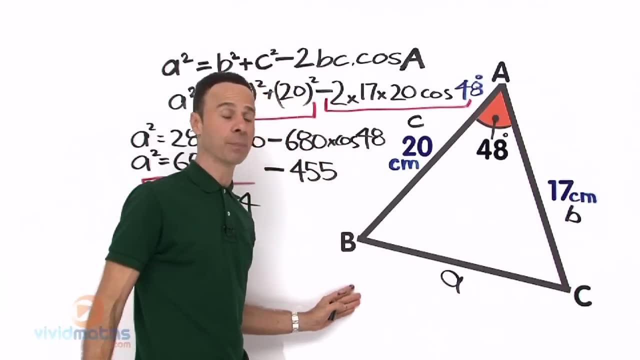 234.. 234.. 234 seems a little big. well, don't forget, it is an A squared. we need to square root both sides. so let us do that Square root, square root. so eventually A is going to equal, which is code for BC. it is the same capital B. capital C is the same as A. so that length. 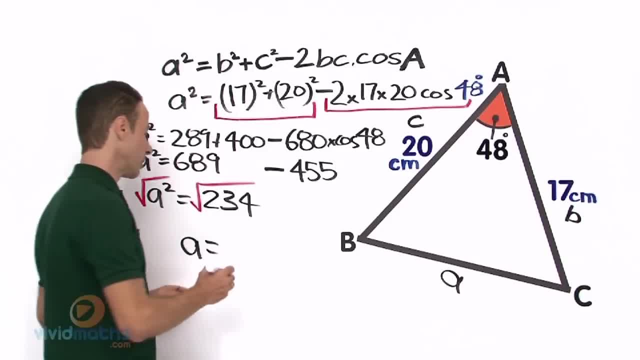 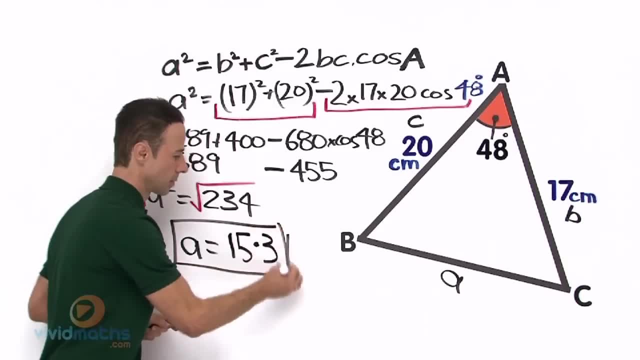 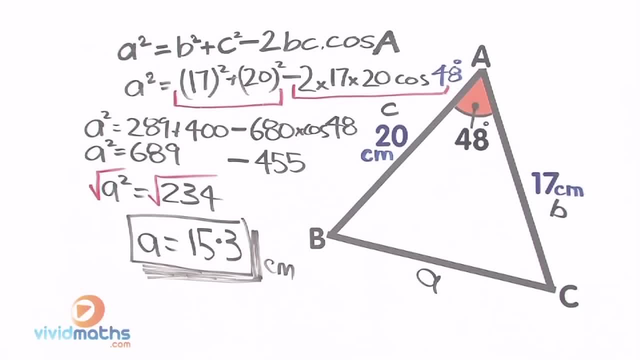 Just keep the number, Not a lot, it is about the same. It's about the same as that. Do the same for all the other ones. Just keep the number and you will be good. That's it. That's it. Thank you for watching. 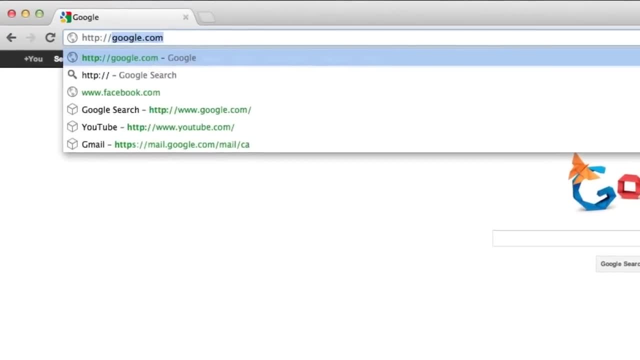 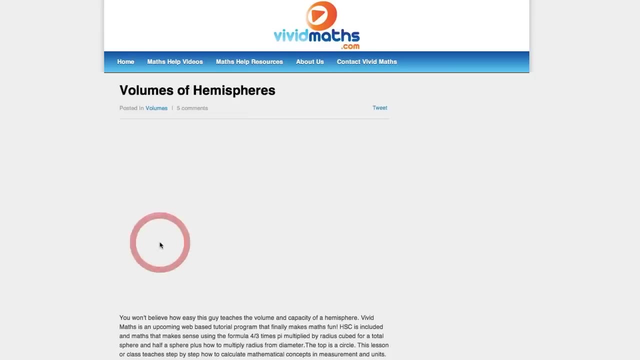 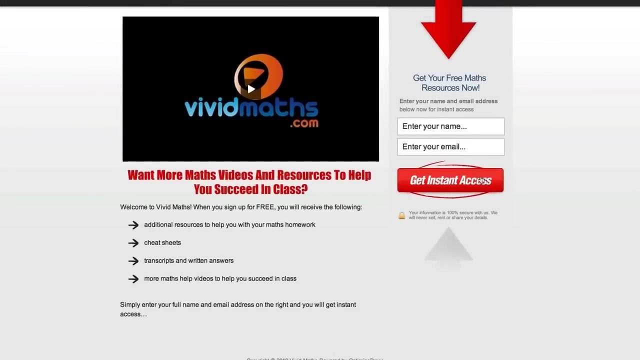 to check out our website at http//wwwvividmathscom. You will find additional resources, cheat sheets, transcripts and other math videos that are not available on Youtube. Lastly, don't forget to subscribe to get access to all the written answers for your math questions plus. other special offers.